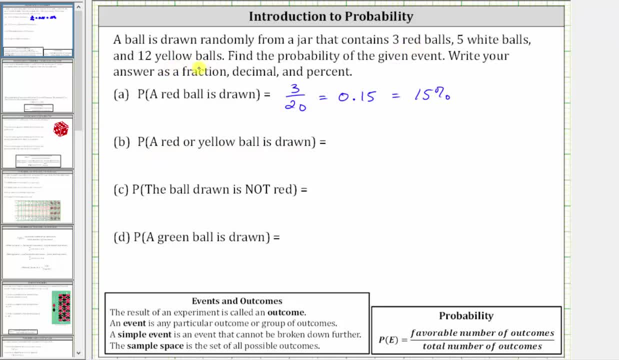 So, because there are three red balls and 12 yellow balls, this time there is a total of three plus 12, or 15 favorable outcomes out of a total of 20 outcomes, And therefore the probability a red or yellow ball is drawn is 15 divided by 20, or 15 20ths. 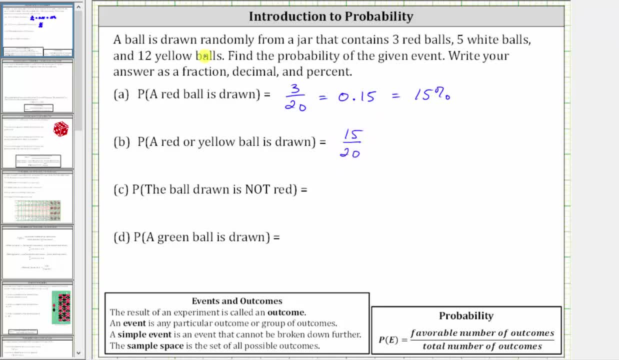 which notice, in this case does simplify, because 15 and 20 share a common factor of five. To simplify, we divide the numerator and denominator by five. 15 divided by five is three. 20 divided by five is four. The simplified probability is 3- 4ths. 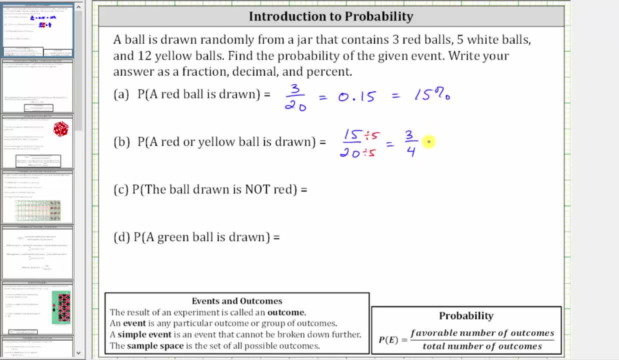 To convert 3 4ths to a decimal, we divide three by four. Three divided by four is equal to 0.75, which as a percentage, is 75%. For part C, we want to find the probability. the ball is not red. 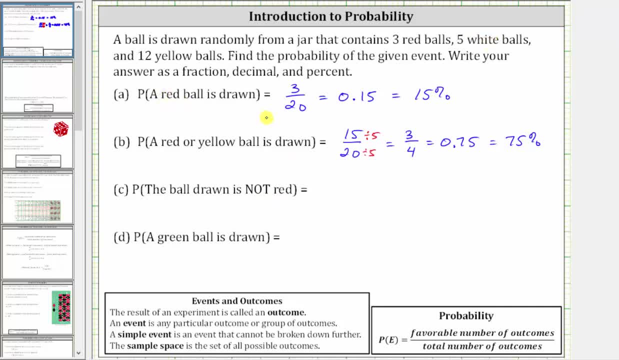 The balls that are not red are the white balls on yellow balls, and because there are five white balls and 12 yellow balls, and five plus 12 is 17,, this time there are 17 favorable outcomes out of a total of 20 outcomes. 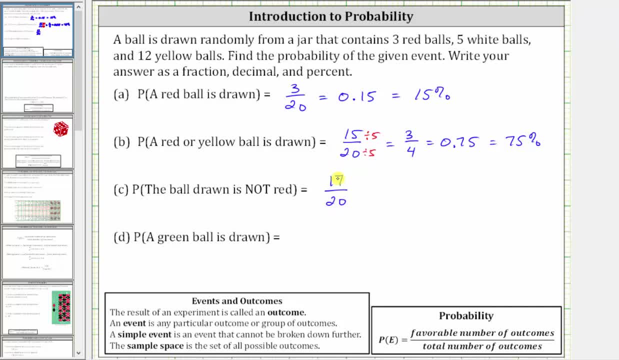 giving us a probability of 17 divided by 20, or 17 20ths, which does not simplify Converting to a decimal: 17 divided by 20 is equal to 0.85, which, as a percentage, is 85%. 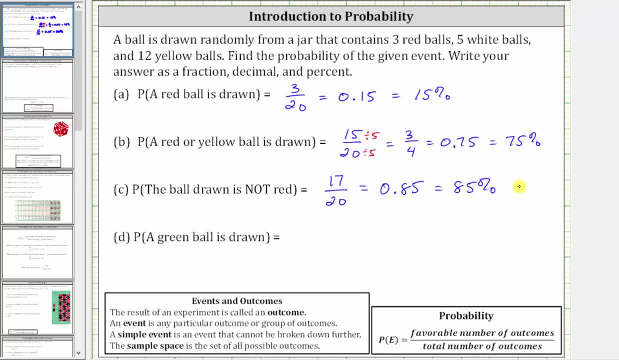 For the last example, we want to find the probability. a green ball is drawn, but notice how there are no green balls in the jar and therefore there are zero favorable outcomes, giving us a probability of zero divided by 20, which simplifies to zero, which is equal to 0%. I hope you found this helpful.